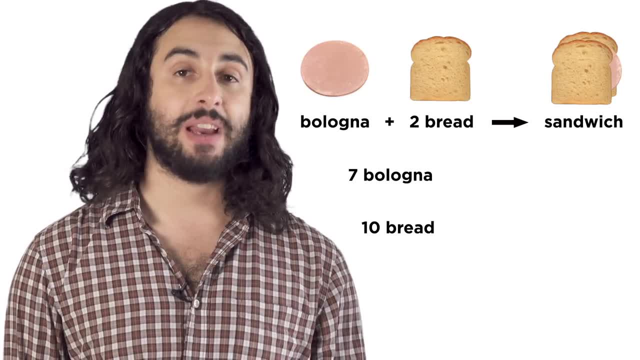 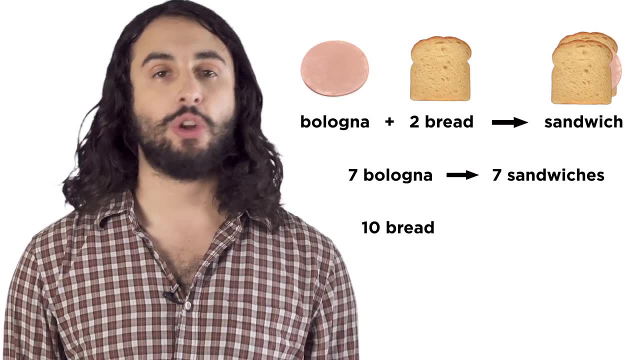 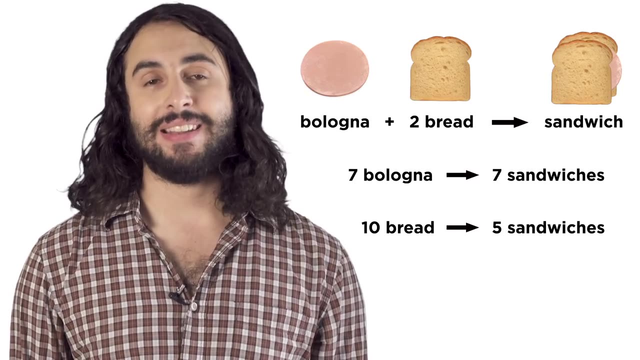 Let's say we have seven bologna and ten bread. How many sandwiches can we make? Well, seven bologna could potentially make seven sandwiches, but ten bread can only make five, because we need two per sandwich. So, even though there's more bread than bologna, it is bread that is the limiting reagent in. 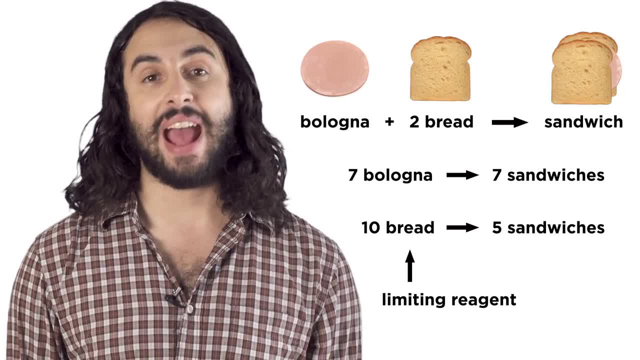 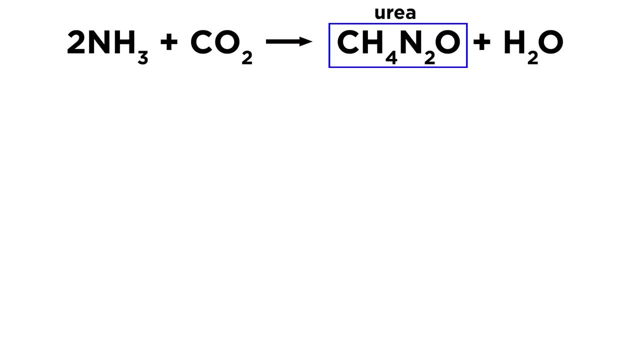 this example, The bread will react fully and leave an excess of two bologna, so bologna is in excess. Let's look at a real reaction. If we start with ten grams of each reactant, which one limits the reaction, Well, the first thing we have to do is convert to moles, because mass doesn't tell us anything. 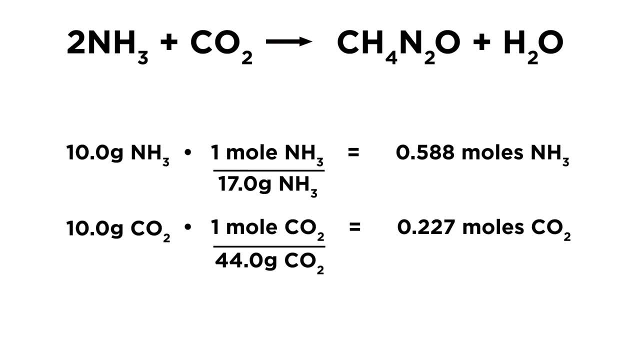 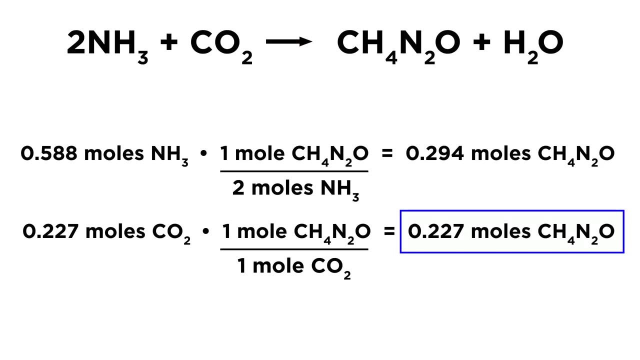 We need numbers, So we convert both to moles using their respective molar masses. We can now look at these numbers a few different ways. One way is to see how many moles of urea each has the potential to produce. Use the stoichiometric ratios to see that CO2 can't produce as much. 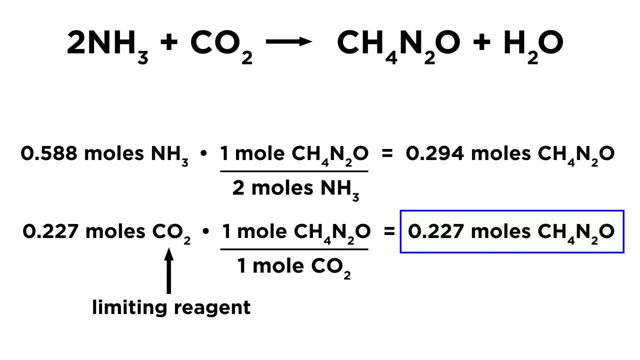 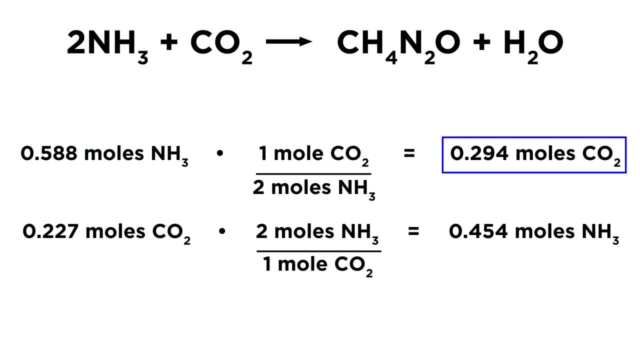 So that must be the limiting reagent. You could also see how much of the other reactant each could react with. This many moles of ammonia could react with this many moles of CO2, which we don't have. This many moles of CO2 could react with this many moles of ammonia, which we do have. 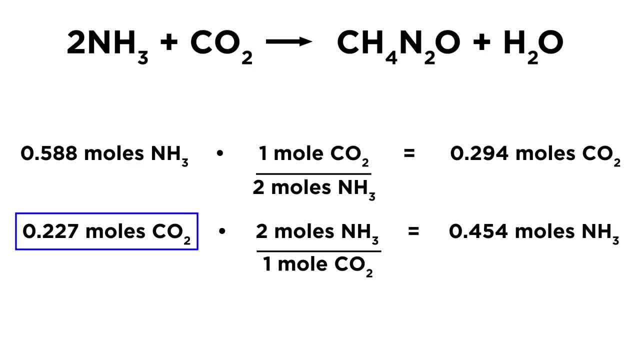 So CO2 will react completely and limit the reaction Once we identify the limiting reagent, we just use the stoichiometric ratios to see how many moles of CO2 each has the potential to produce. We can now look at this one. 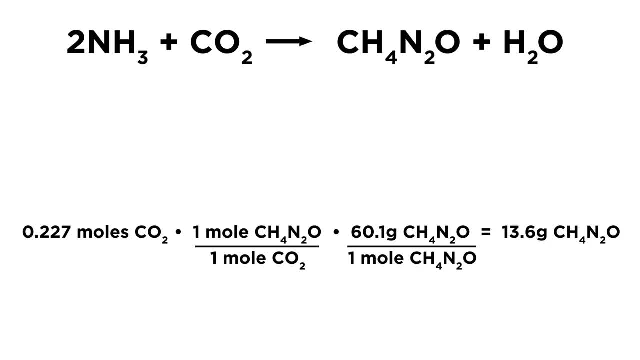 We just use the data for that substance to calculate how much product we will get, since that substance will get used up. If we used the other one, we would get the wrong answer, because not all of the reagent in excess will go towards generating product. 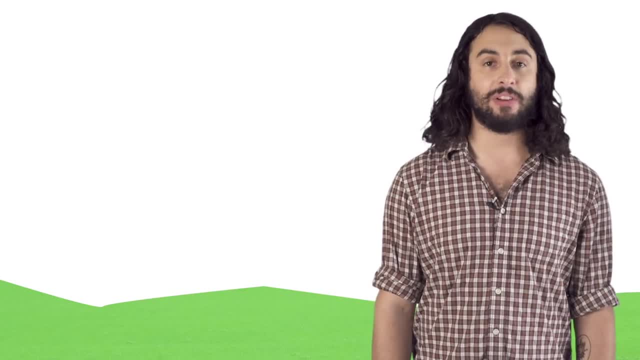 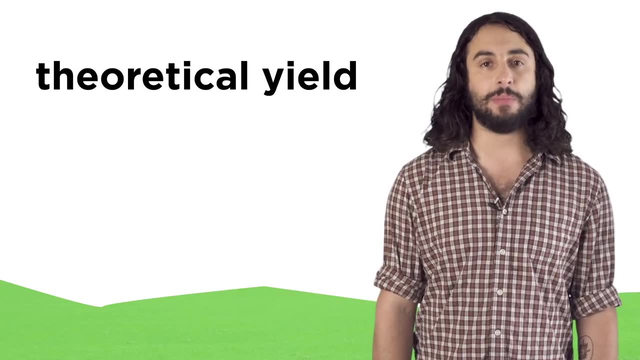 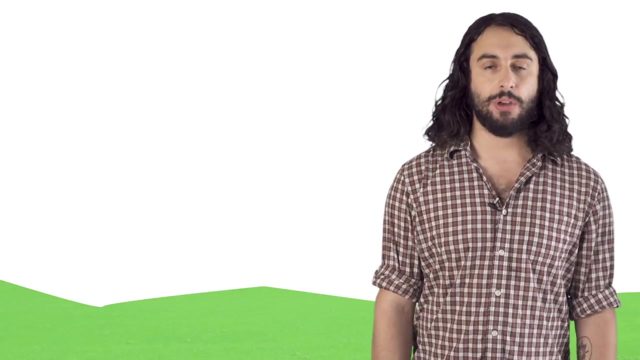 Another real-life limitation of chemistry is that the amount of product we calculate that we should get is actually just the theoretical yield. This is the amount of product we can expect if every molecule of reactant can produce. In reality, this does not occur and the actual yield will always be some fraction of the